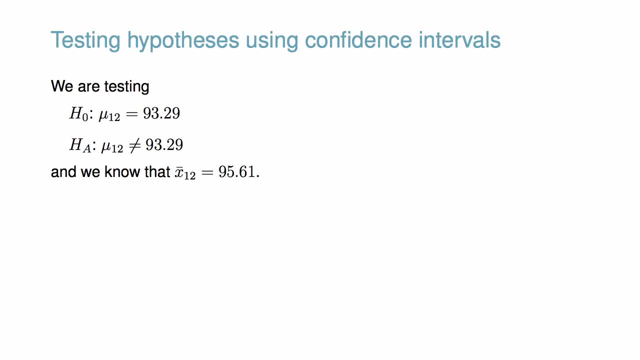 We can start the evaluation of the hypotheses by comparing the 2006 and 2012 run times using a point estimate from the sample. The sample mean is 95.61 minutes. This estimate suggests the average time is actually longer than the 2006 time: 93.29 minutes. 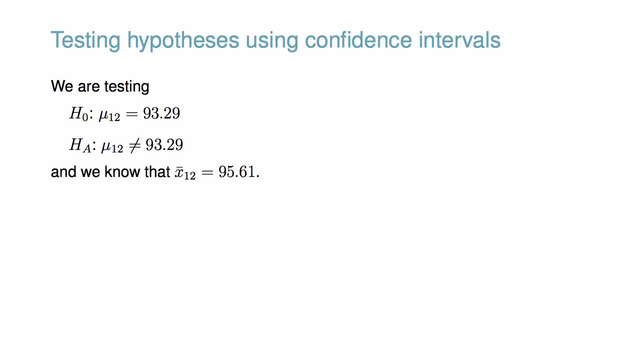 However, to evaluate whether this provides strong evidence that there has been a change, we must consider the uncertainty associated with the sample mean. A confidence interval provides a range of plausible values for the population mean Based on the data. a 95% confidence interval for the 2012 population mean was calculated as 92.45 to 93.29 minutes. 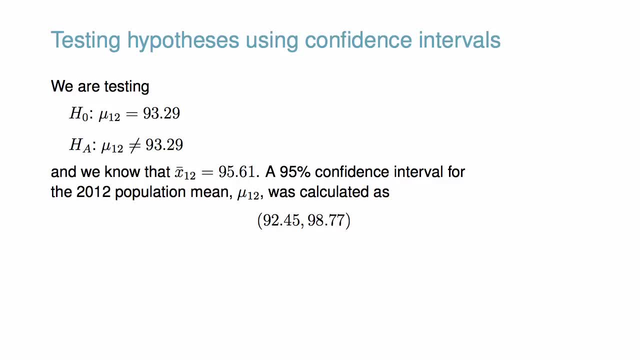 Based on the data, a 95% confidence interval for the 2012 population mean was calculated as 92.45 to 93.29 minutes. Based on the data, a 95% confidence interval for the 2012 population mean was calculated as 92.45 to 93.29 minutes. 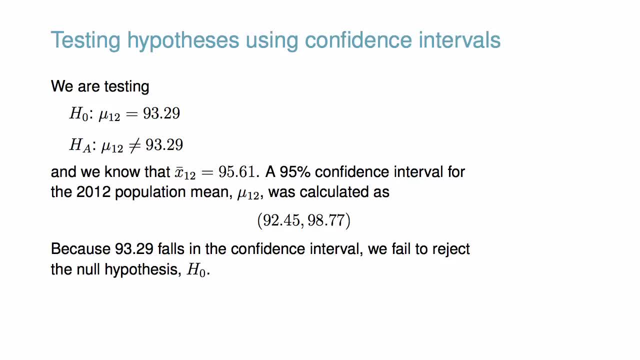 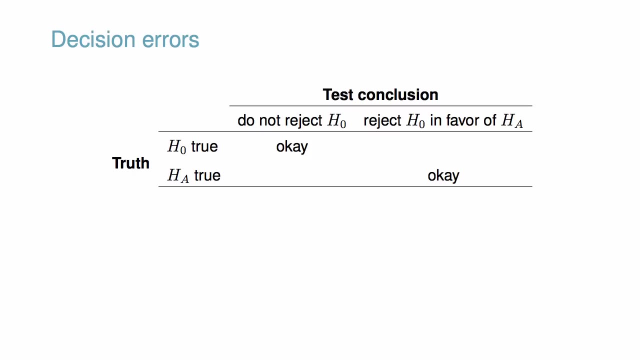 Because the 2006 mean of 93.29 falls in the range of plausible values for the true mean race time in 2012,. we cannot say the null hypothesis is implausible, That is, we fail to reject the null hypothesis. Hypothesis tests are not flawless. 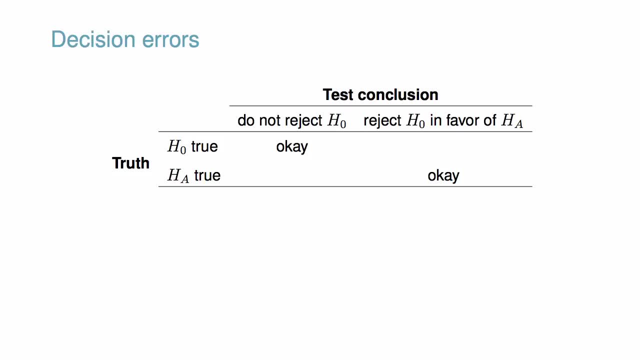 In a hypothesis test, we make a statement about which of the null or alternative hypotheses might be true, but we may choose incorrectly. There are four possible scenarios in a hypothesis test. Two scenarios represent a correct decision and two scenarios represent an error. A type 1 error is rejecting the null hypothesis when the null hypothesis is actually true. 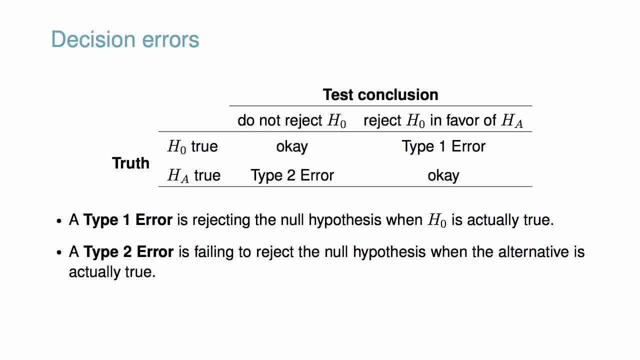 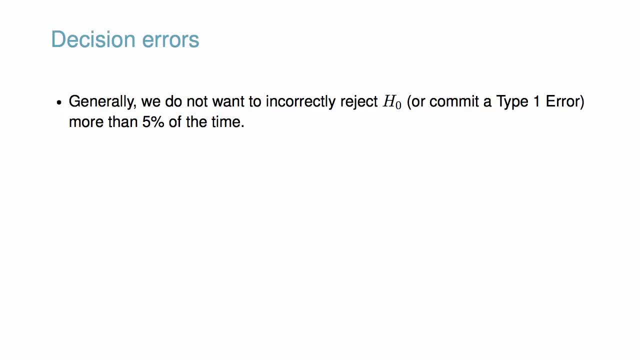 A type 2 error is failing to reject the null hypothesis when the alternative is actually true. Generally, we do not want to incorrectly reject the null hypothesis more than 5% of the time. This corresponds to a significance level of 0.05, denoted by the alpha. 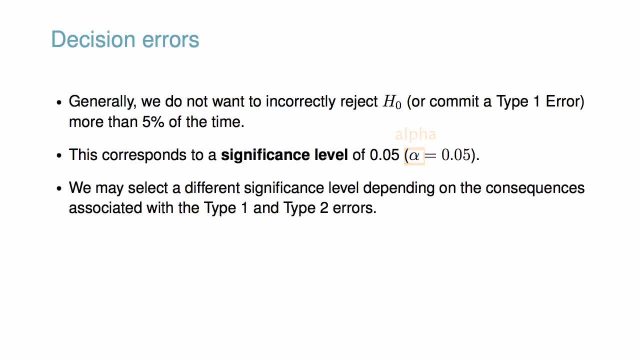 This corresponds to a significance level of 0.05, denoted by the alpha. We may select a different significance level depending on the consequences associated with type 1 and type 2 errors. However, reducing our chances of one error increases the chances of the other error. 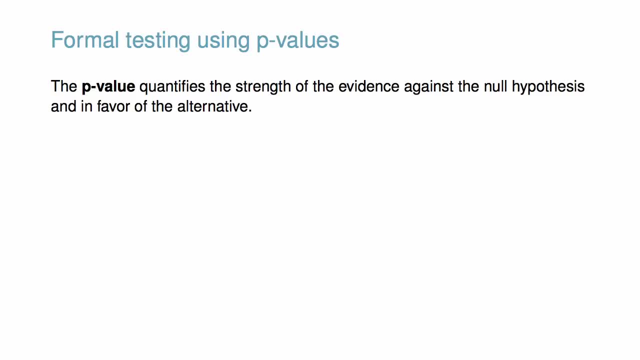 The p-value is a way of quantifying the strength of evidence against the null hypothesis and in favor of the alternative. The p-value is the probability of observing data at least as favorable to the alternative hypothesis as our current data set, if the null hypothesis is actually true. 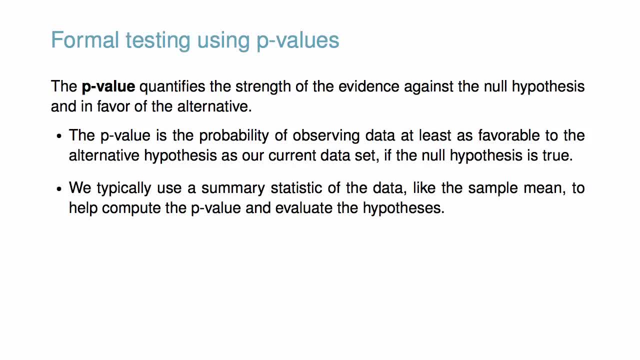 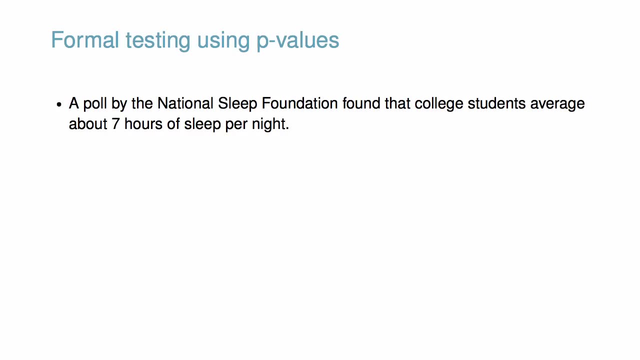 If the null hypothesis is actually true. We typically use a summary statistic of the data, like the sample mean, to help compute the p-value and evaluate the hypotheses. We evaluate the hypotheses by comparing the p-value to the significance level, usually 0.05.. 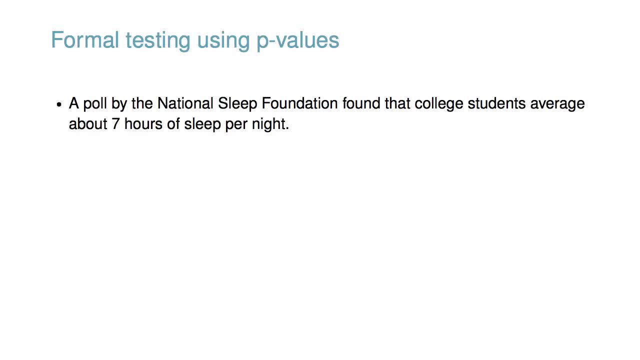 Let's do an example. A poll by the National Sleep Foundation found that college students average about 7 hours of sleep per night. Researchers at a rural school test the claim that their students are sleeping longer than the national average with a one-sided alternative hypothesis. 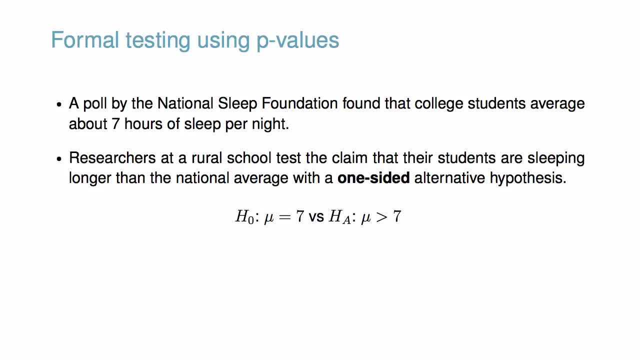 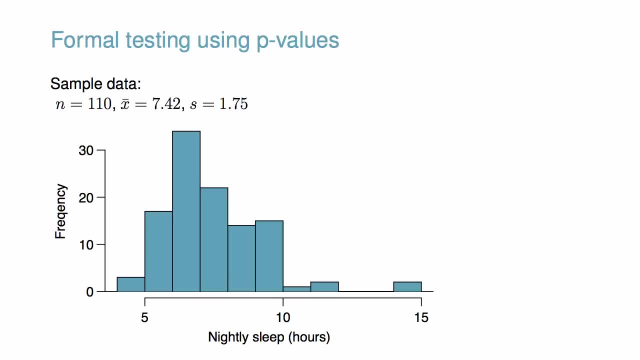 The null hypothesis is that the true mean hours of sleep equals 7, and the alternative hypothesis is that the true mean hours of sleep is greater than 7.. The researchers conducted a simple random sample of 110 students and found that these students averaged 7.42 hours of sleep, with a standard deviation of 1.75 hours. 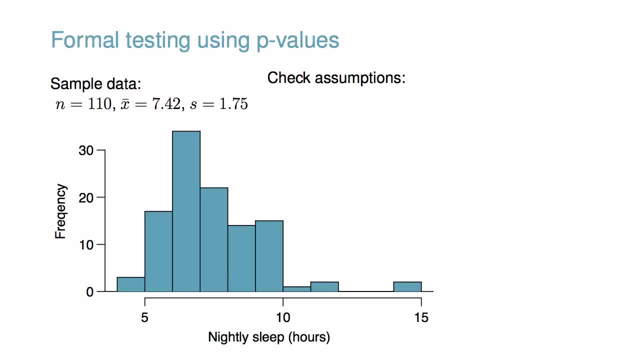 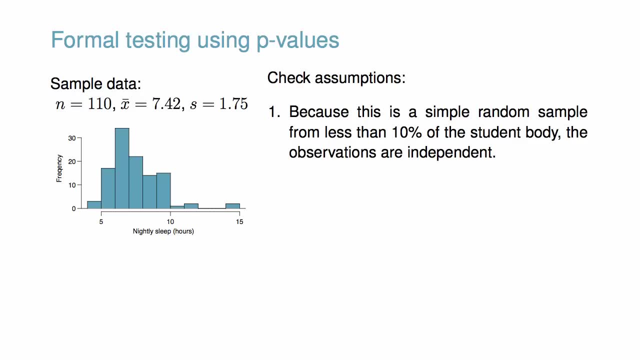 To proceed with hypothesis testing, we first need to evaluate if the normal model is valid for the sample mean. First, because this is a simple random sample from less than 10% of the student body, the observations are independent. Second, the sample size in the sleep study is sufficiently large, since it is greater than 30.. 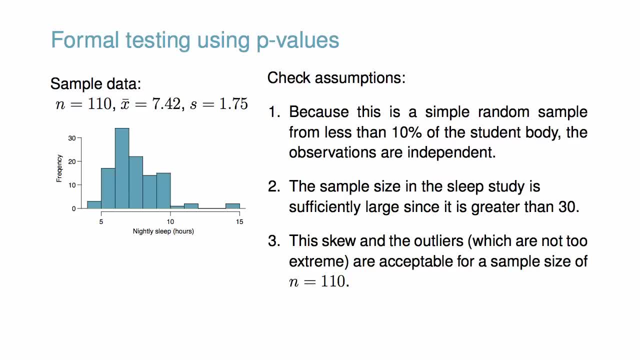 Third, although the data share moderate skew in the histogram and the presence of a couple of outliers, it is not too extreme and are acceptable for a sample size of 110.. With these conditions verified, the normal model can be safely applied to the sample mean. 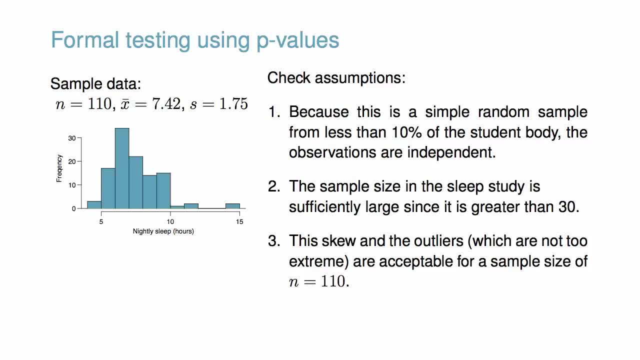 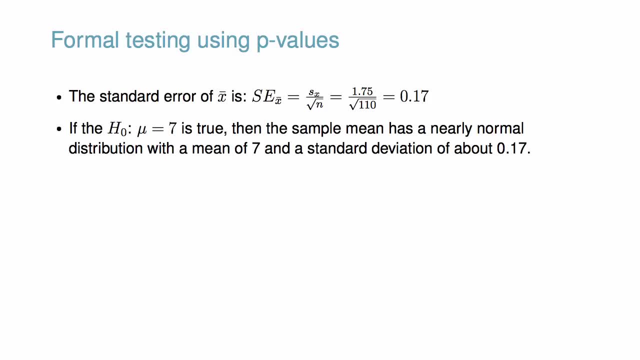 and the estimated standard error will be accurate. The standard error of the sample mean is calculated to be 0.17.. If the null hypothesis is true, then the sample mean has a nearly normal distribution, with a mean of 7 and a standard deviation of about 0.17.. 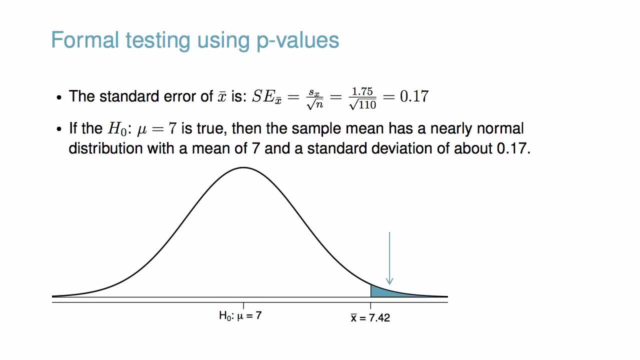 The shaded tail represents the p-value, which is the chance of observing such a large mean, conditional on the null hypothesis being true. We compute the p-value by finding the tail area of this normal distribution. First, compute the z-score of the sample mean. 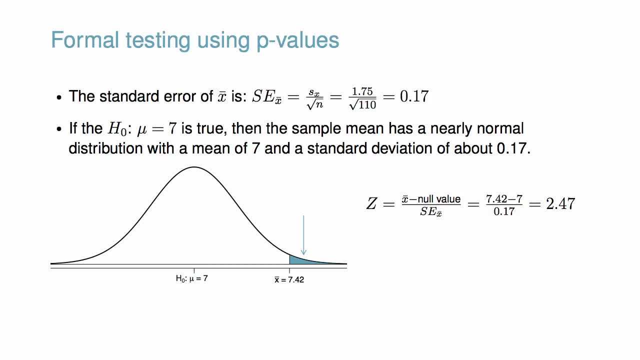 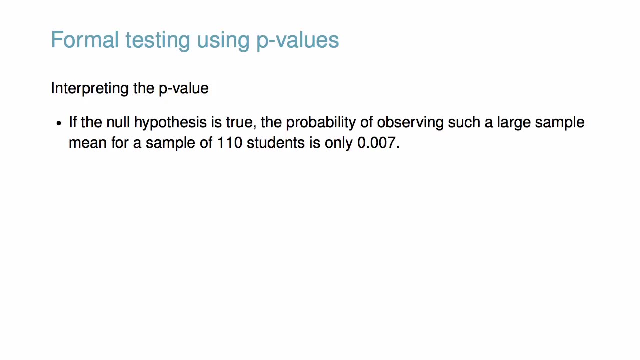 which is 2.47.. Then use the normal probability table to find the shaded area, which is 0.007.. This is the p-value. If the null hypothesis is true, the probability of observing such a large sample mean for a sample of 110 students is only 0.007.. 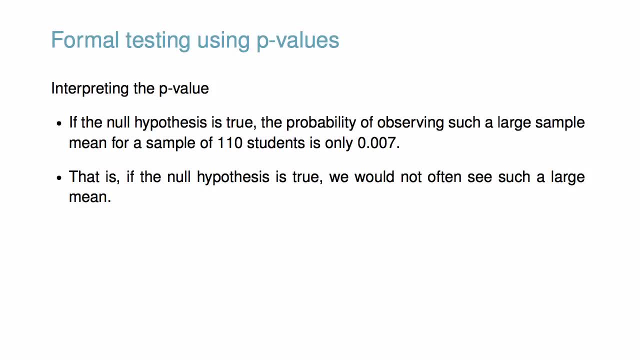 That is, if the null hypothesis is true, we would not often see such a large mean. We evaluate the hypotheses by comparing the p-value to the significance level, Because the p-value is less than the significance level of alpha equal to 0.05,. 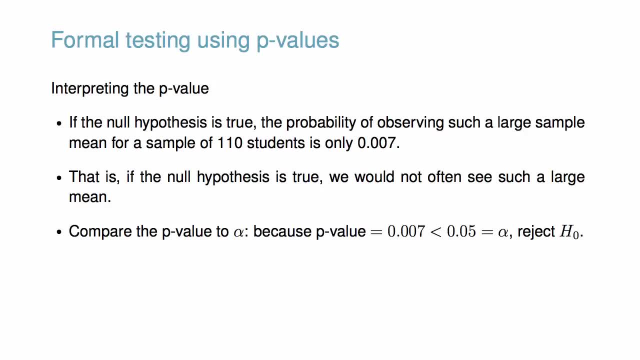 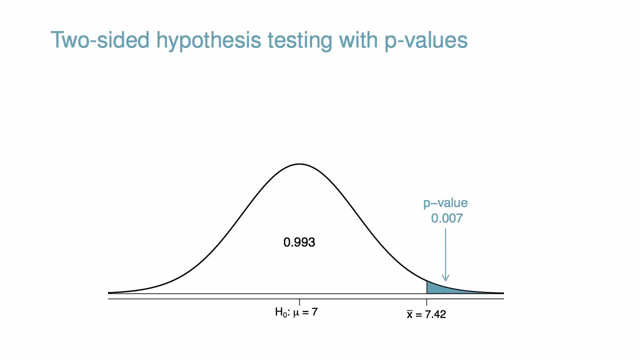 we reject the null hypothesis. What we observed is so unusual with respect to the null hypothesis that it casts doubt on the null hypothesis and provides strong evidence favoring the alternative. Before, with a one-sided test, we shaded the single tail in the direction of the alternative hypothesis. 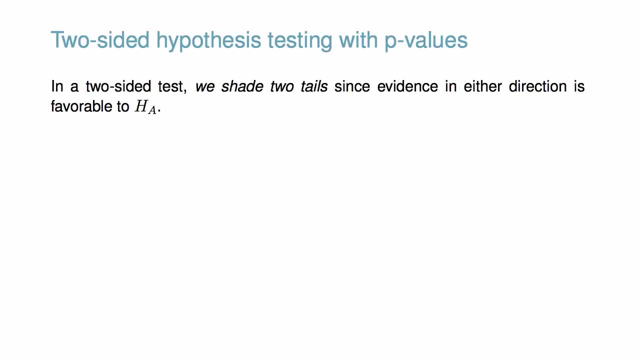 to calculate the p-value In a two-sided test, we shade two tails, since evidence in either direction is favorable to the alternative hypothesis. Let's consider the hours of sleep example again, but this time with a two-sided alternative hypothesis. That is, the population mean is not equal to 7.. 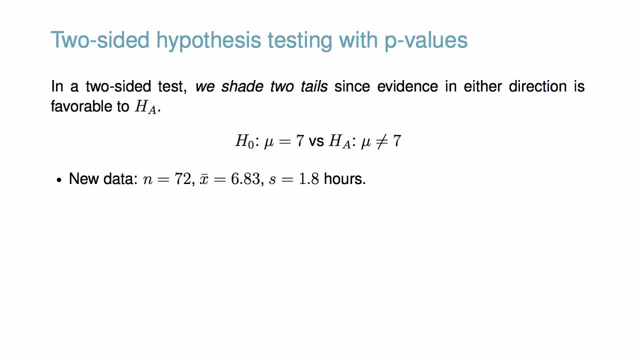 Sample data are collected at a different college, where 72 students averaged 6.83 hours of sleep, with a standard deviation of 1.8.. First verify assumptions and then proceed with the p-value calculation. Here the alternative hypothesis is two-sided. 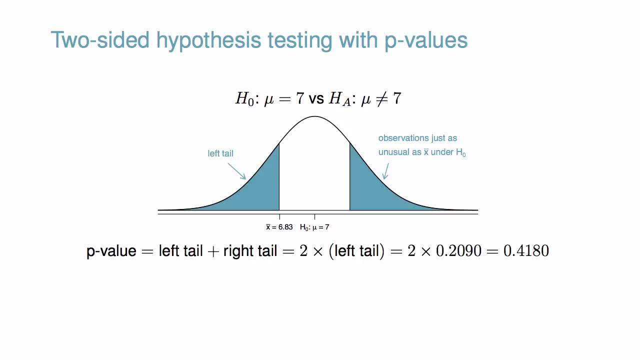 so both tails must be shaded for the p-value. The p-value can be calculated as a left tail plus the right tail or as 2 times the area in a single tail, which yields a p-value of 0.4180.. This p-value is relatively large, and it is larger than the 0.05 significance level. 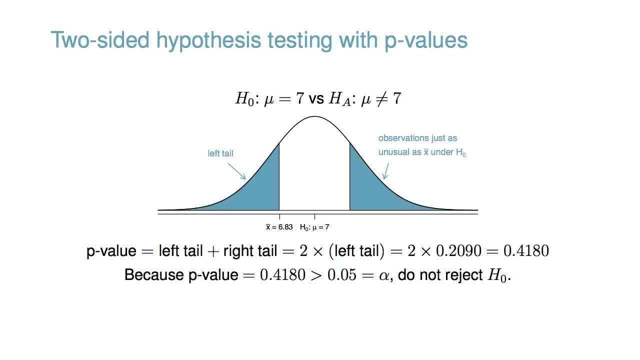 so we should not reject the null hypothesis. That is, if the null hypothesis is true, it would not be very unusual to see a sample mean this far from 7 hours and possibly do a sampling variation. Thus, we do not have sufficient evidence to conclude. 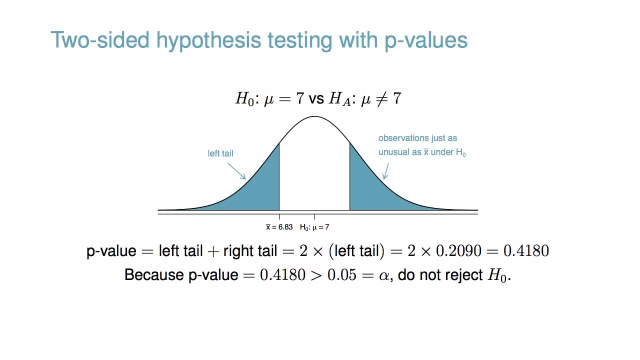 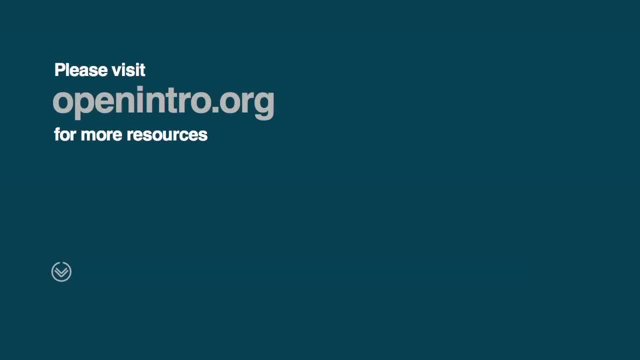 that the true mean hours of sleep in this college is different than 7 hours. In this video, we introduced hypothesis testing. If you learned something you found interesting, share this video with a friend and visit openintroorg for more resources.